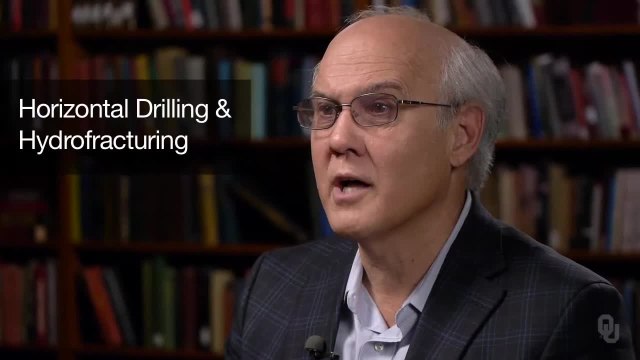 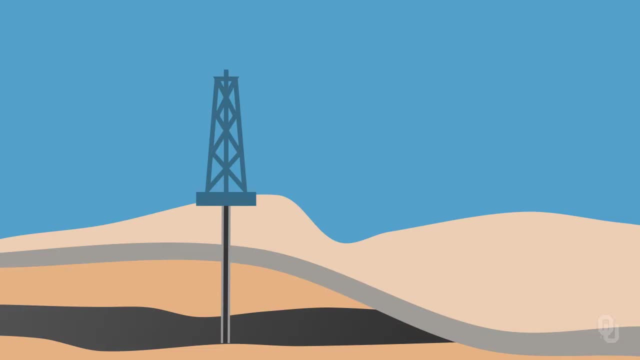 Related to these shale gas reservoirs is horizontal drilling and hydro fracturing. Twenty years ago, if you wanted to drill a well, you would drill a vertical well and you would intersect, let's say, a 100-meter unit of rock that you could extract hydrocarbons from. 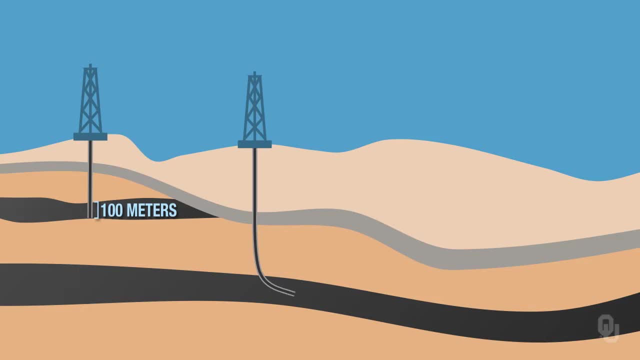 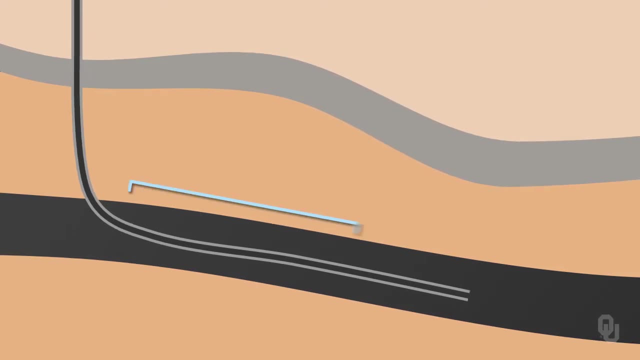 But now what happens is we can drill horizontally, You drill down and you drill down, And then you drill laterally, So you can drill through a reservoir unit for miles, so you can encounter a lot more of the rock and therefore extract a lot more hydrocarbons. 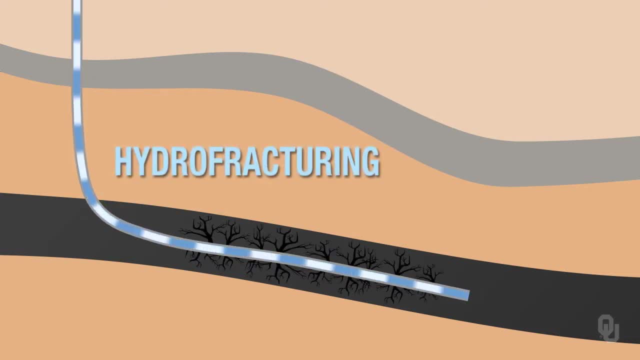 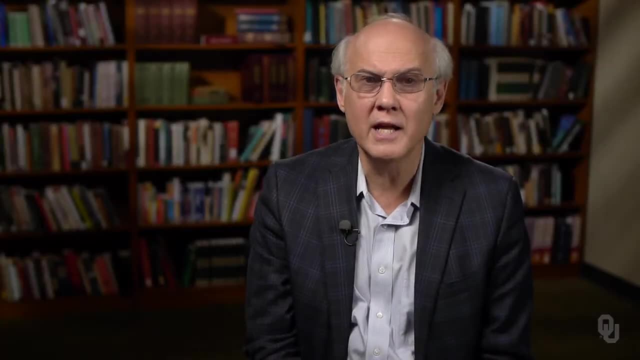 The oil companies use hydro fracturing to break the rocks up and that allows more gas and oil to be extracted. This has been a major change in the oil business because unproductive units which didn't have a lot of porosity and permeability 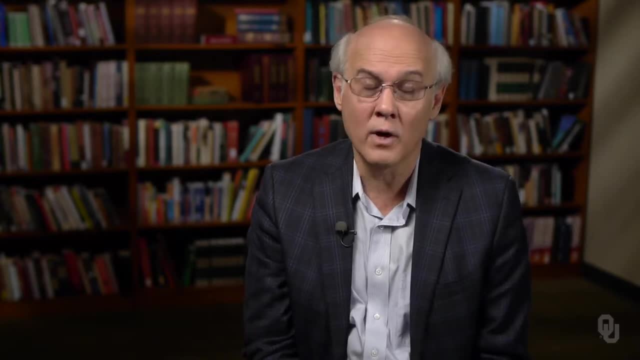 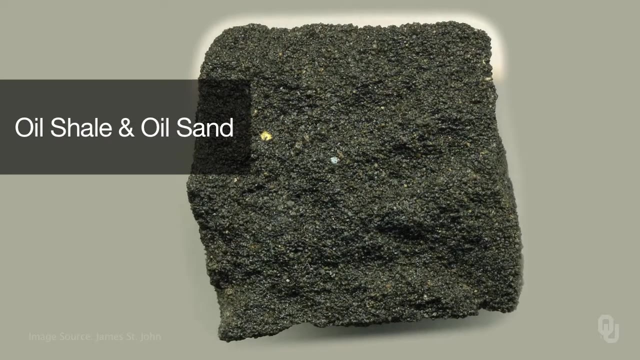 and couldn't produce much oil and gas. now we can get oil and gas out of them because of horizontal drilling and hydro fracturing. Another type of fossil fuel will be oil shales and oil sand, For example. there are major deposits of oil sands in Canada. So what are some of the negatives with extracting fossil fuels? We mentioned a few for coal already, but for hydrocarbons you have oil spills, which can be a major problem. Another issue is injection of wastewater, which can produce earthquakes, And then there's CO2 release, which can influence global warming. 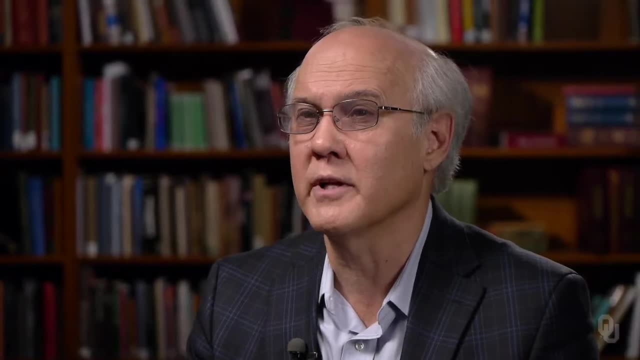 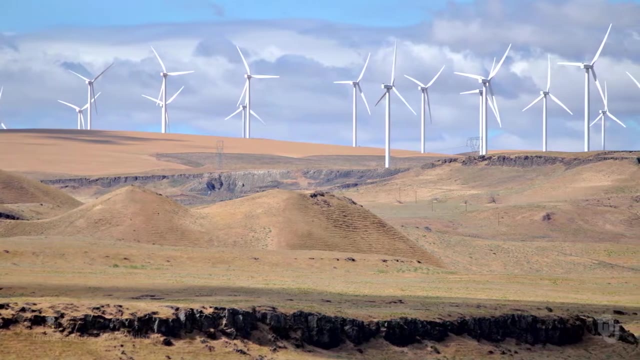 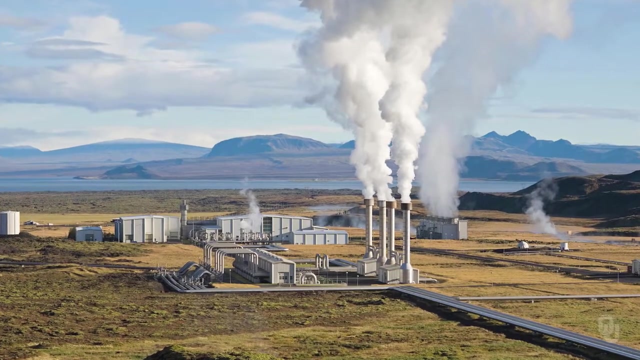 What about other energy sources, like renewable energy sources? Perhaps many of you have noticed there are many, many new wind farms all over the Midwest. Those produce a lot of energy. Another source is geothermal energy. That's hot rock underground. It can heat rocks up. 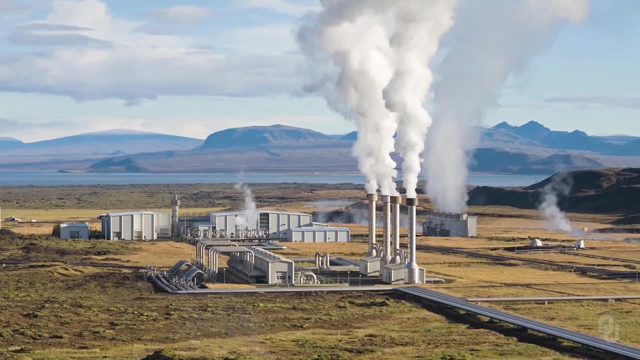 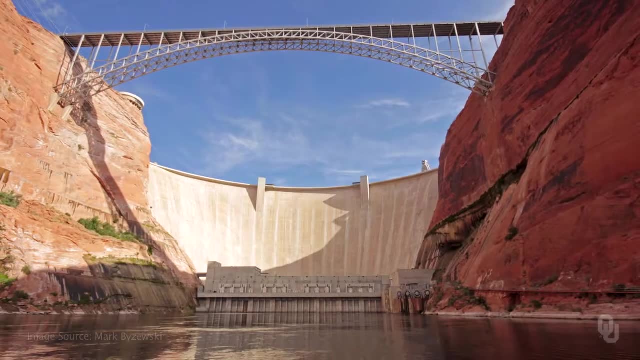 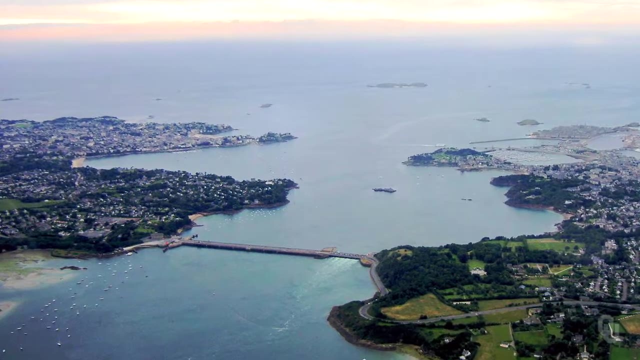 And you can put water down there and you can produce energy from that. Hydroelectric power provides 15% of electricity in the United States today. on major rivers like the Colorado, Tides can be another source of energy. We currently don't have any plants in the United States that use tides, but there are some around the world. 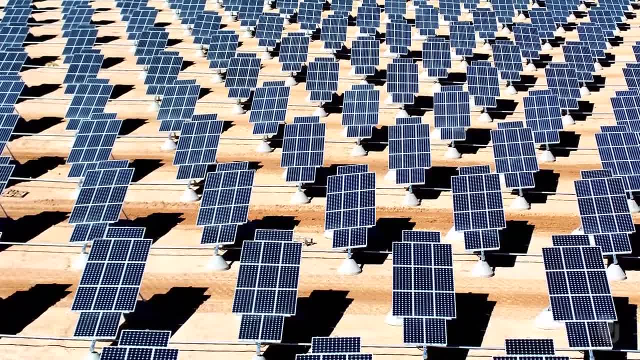 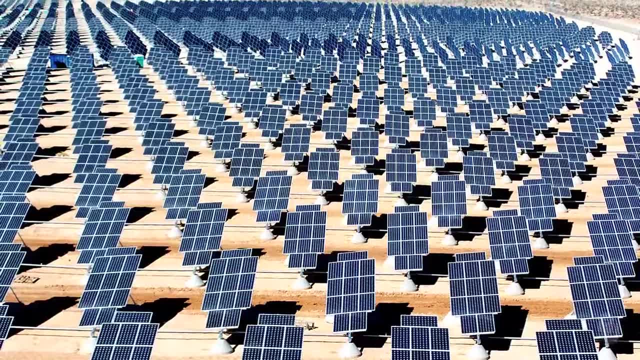 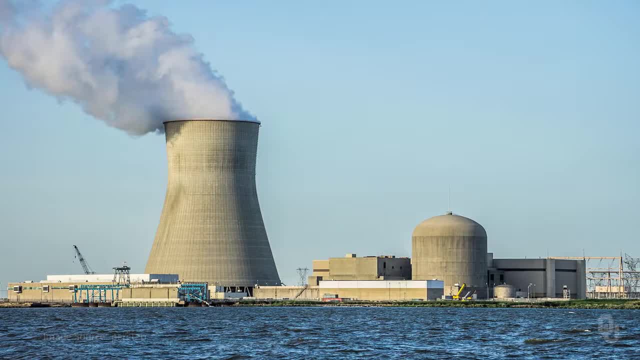 Solar energy is gaining popularity, particularly as the costs for solar energy have come down. It will probably not be a major factor, however, for many decades, And we have fission and perhaps fusion power plants. Our current nuclear power plants are fission power plants. 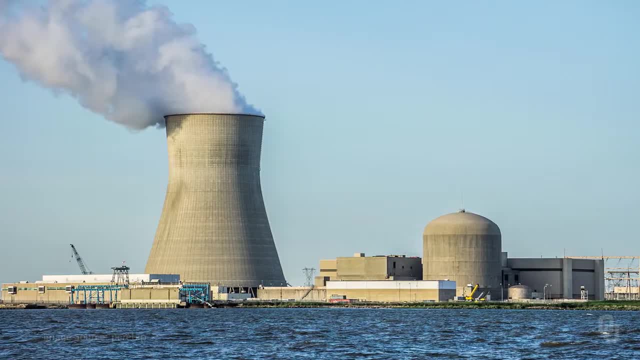 And perhaps we will have fusion power plants in the future.